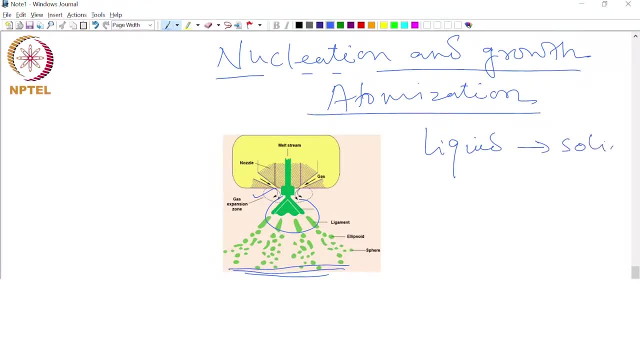 is how this solid is going to exchange into a greater particle. right, So it12 confrontation is involved in this process, right, And this is a very important aspect that we need to understand as to you know how these solidification happens in these process and you know what are the different attributes of this and you know what. is the process during solidification. So that is the�� this process taken and a 3 point shift anywhere will also lead to 1900 and this solidification is involved. So to respond, a more frequent coating part of the material Right, So it is called the constant load acceleration. the time will also take a nine minutes. Now we are going to move to second phase. this process will be moving through the Wyoming pine and theitt- and what one. we do it up here, you know, next to the soil. tweektent publination already Right, you know how to easily materialize the solid derivative. 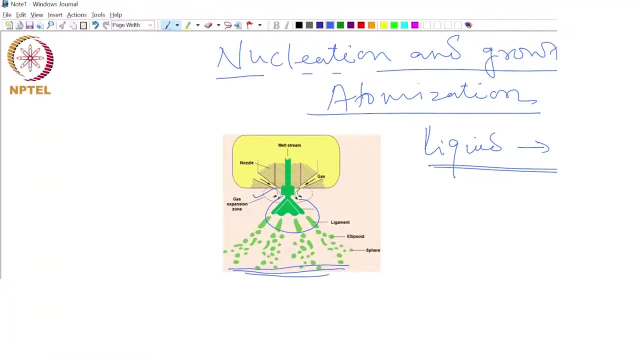 you know what are the details of that and so on. So that is, that is what we are going to learn in in this class today. ok, So solidification, or the liquid to solid transformation, can be understood from this concept called nucleation and growth. Nucleation is nothing but you. 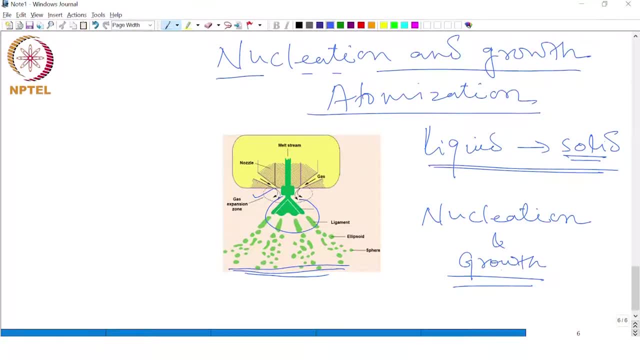 know, the formation of the first solid particles. if you talk about the liquid to solid transformation, For that matter, it is true for any other transformation also. The product phase, the formation of the product phase. the first very particle of the product phase that forms from the parent phase is called a nucleus. ok, So that is the starting. 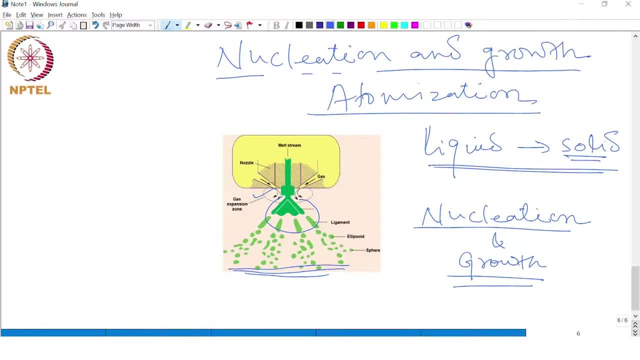 of the transformation. So in this case, when it is transforming from liquid to solid, the nucleus is the, the first, the very first tiny particle of the solid that gets transformed from the, The liquid phase, as you cool it down below the melting point, right, So above the melting. 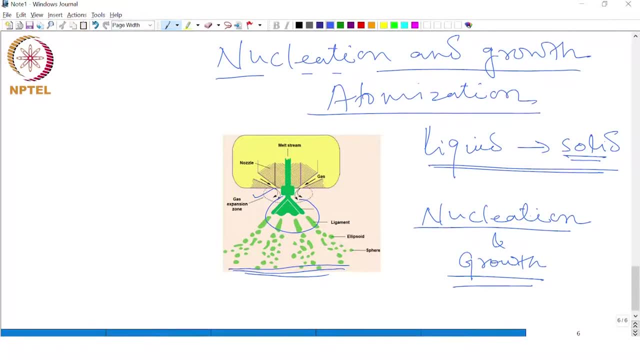 point you have the liquid. because the liquid is more stable above the melting point in those kind of temperatures, and as you cool it down the solid becomes more stable. right, So the stability of any state of matter that depends on its energy? right? Because it is. 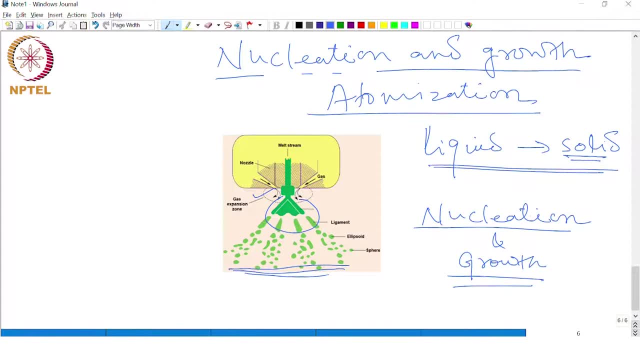 because any matter would like to stay at the minimum energy level, right? So when you see a matter in a particular state under particular conditions, it means that under those conditions it is existing in that particular state because that state will give the material or the system the lowest energy. ok, For example, if you 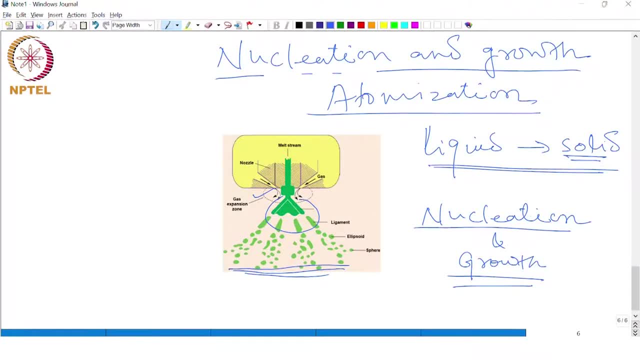 Force of a proton, The flux of a proton, The flux in whom? The flux in whom? sea water, as we all see, water. it is liquid in room temperature and atmospheric pressure. right, So that tells you that the water in liquid condition is the is the most stable phase in. 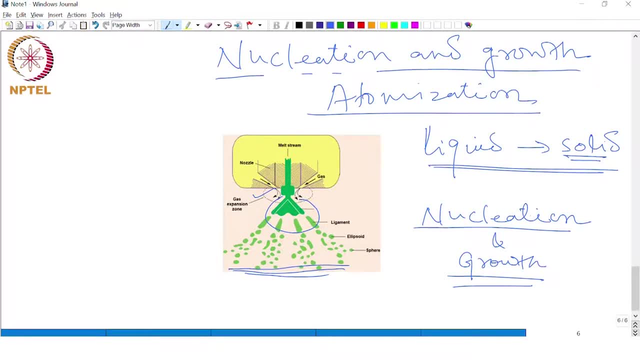 room temperature and atmospheric pressure, because that particular state will give it the minimum energy. So it will be in the lowest possible energy state in room temperature and atmospheric pressure and that is why it is. the liquid form of water is stable in room temperature and we always see it in the liquid form, generally right at room temperature. 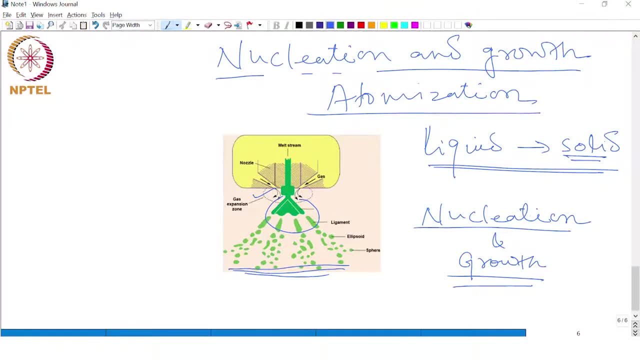 So, unless otherwise it is cooled down below the melting point, it is frozen below 0 degree centigrade. you know it is going to remain liquid, right? And if you want to change the state then you will have to do something to the system. that means you need to do certain work to the system in terms of 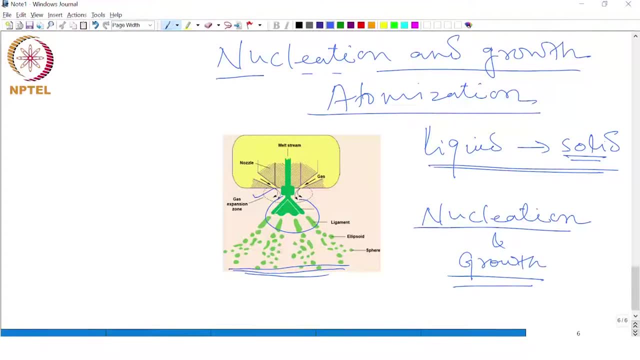 either extraction of it or addition of it. ok, So all this, you know, boils down to the energy of the system. You can also call it the internal energy of any material or system- And whether a particular state of a matter will transform to another state. 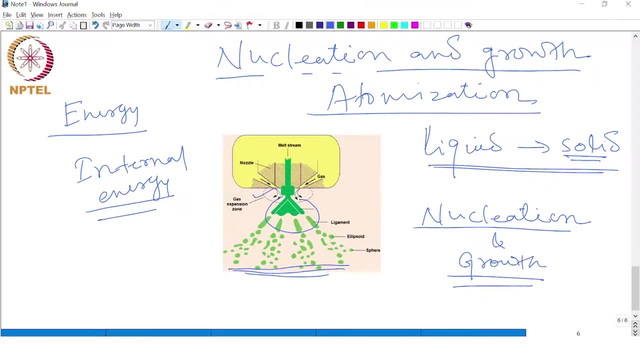 that would depend on whether the energy is getting reduced or not. ok, So, for example, any material will go from liquid to solid if going into the solid reduces the energy of the material, right? So whenever you have a transformation like this, it will happen only when the energy is. 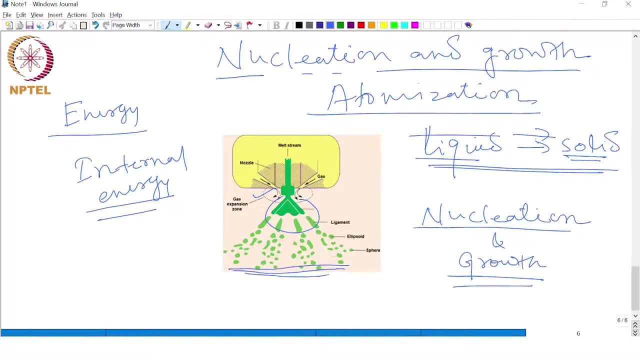 reducing ok. So that particular aspect is described in terms of a particular energy known as Gibbs free energy or free energy. This is actually related to the internal energy of the system of the material. This is generally denoted as chi ok. So change in the Gibbs free energy will decide whether the transformation will. 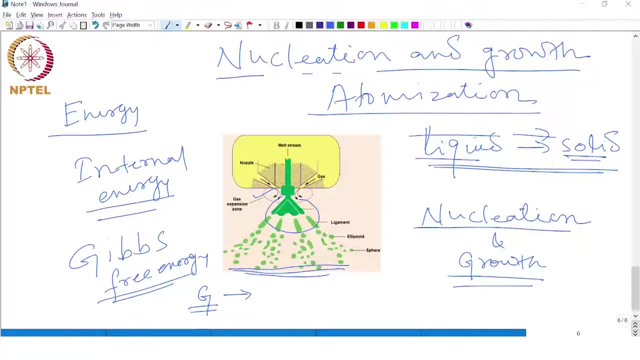 proceed or not. That means when it is changing from the parent phase to the product phase or from the parent state to the product state, whether this energy is reducing or not, In other words, the change from going from state 1 to state 2,. 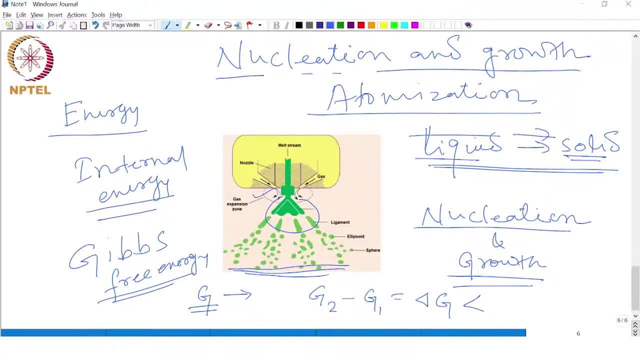 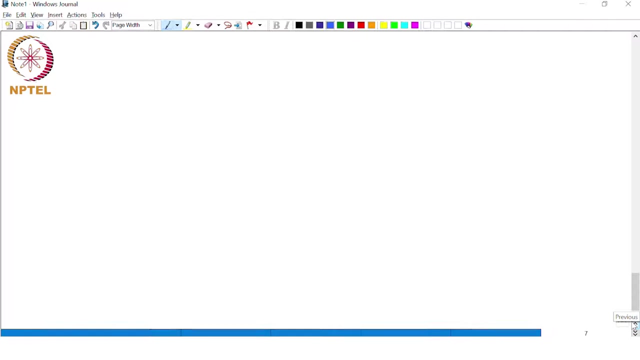 this delta G whether it is negative or not. ok So. So a transformation will happen or will proceed in the forward direction only when the delta g is negative. ok, So, as far as the liquid to solid transformation is concerned, this free energy change can be explained with the help of a diagram like this: 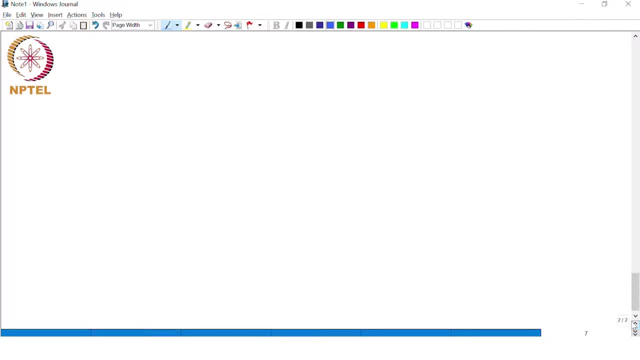 Here you have the free energy on the y axis and temperature on the x axis. Now again taking the same transformational liquid to solid. ok, 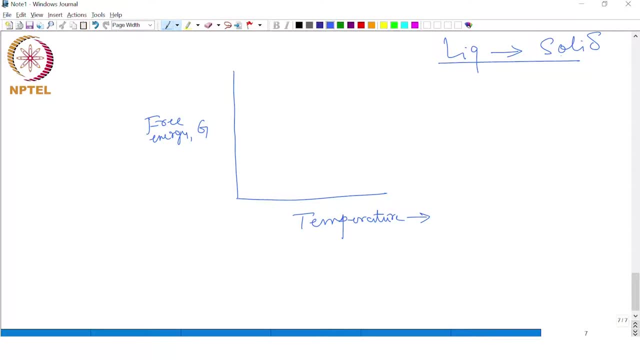 Thank you. So this is the melting point that we denote as Tm. all right, So here you can see these two curves that you have. they represent the free energy of the solid and the liquid as a function of temperature. This one is for the solid: gs. ok, that is, free energy of the. 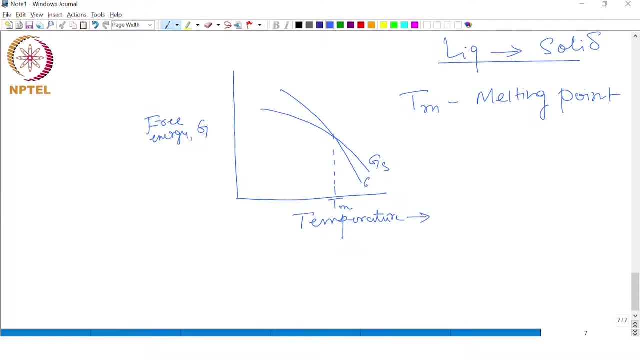 solid and this one is the free energy for the liquid, denoted as gl. ok, So now you can look at these curves on the left and right of the melting point Tm. that means, if you come to This or that side, what do you see in the free energies? ok, So above the melting point. 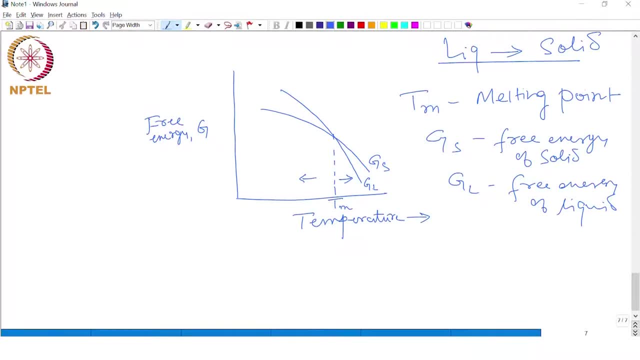 you can see, the free energy of the liquid is lower than that of the solid. ok, So this is why, and therefore the liquid is more stable above the melting point and that is why it melts as you cross themelting temperature and becomes liquid right Similarly below. 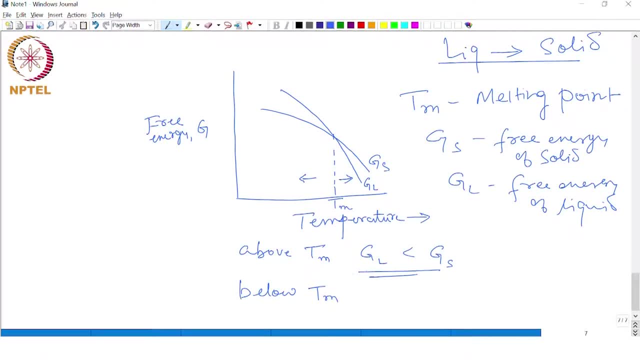 Tm is less than that of the liquid and therefore the solid is more stable below the melting point, and that is why, when you reduce the temperature below the melting point, the liquid turns into a solid right. So therefore you need to see this change in the free energy. 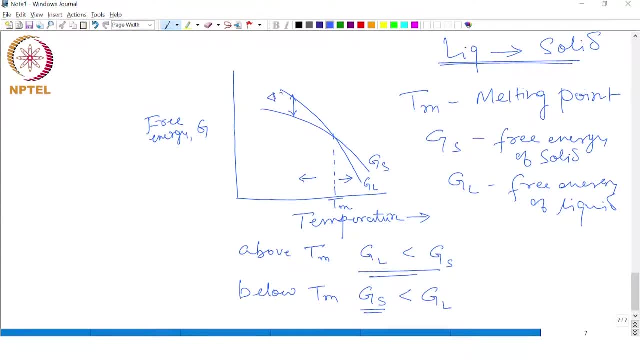 delta G and below the T m, you see that G s is less than G L. So if you take the delta G, That becomes negative below the melting point. ok, as you reduce the temperature and bring it down, the solid will have lower free energy compared to liquid. as a result, delta G is 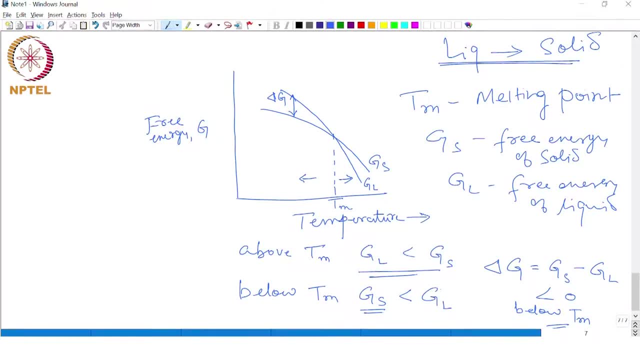 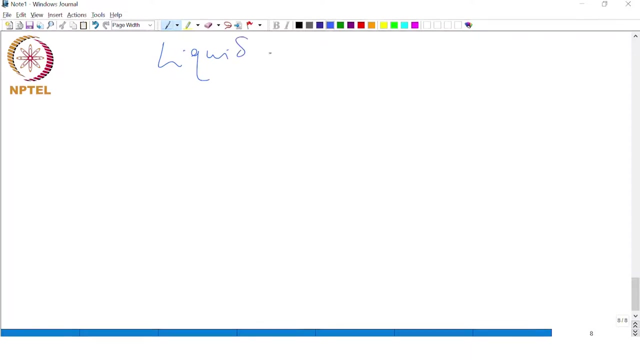 negative. So when you cool it down below the melting point, this liquid to solid transformation takes place right, So that you can see with the help of this particular diagram. ok, Now, In the solid forms it does not form at once the solidification or the formation of the 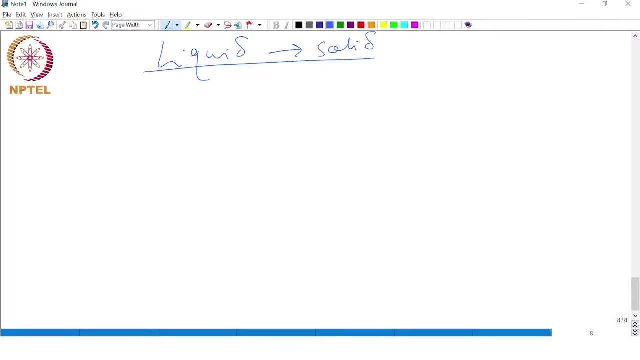 solid particles. it starts with a very small, tiny particle, as I said before, the the very first particle that It forms as you cool it down below the melting point, So that is known as the nucleus. and then, if this, this small particle, this tiny particles, if it attains a size which 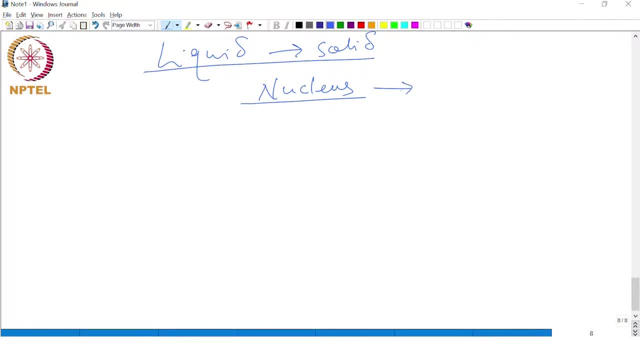 is stable under those conditions, when it is solidifying from the liquid to the solid in that particular atmosphere in the liquid. If this small particle is stable, then it will grow ok. So that is what is the growth process, when more and more atoms will join these tiny. 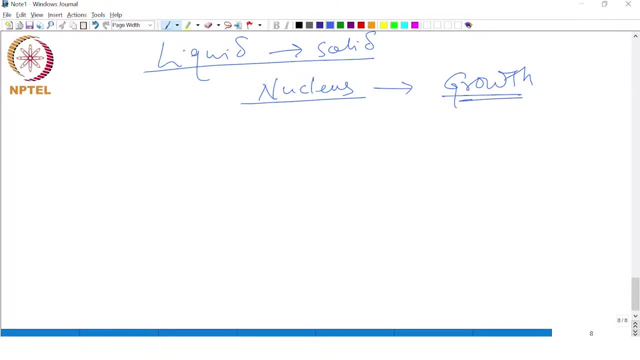 nucleus and it will continue to grow. and finally, you know, this solid material will grow from the liquid Right. So the free energy change that we talked about, the delta G, 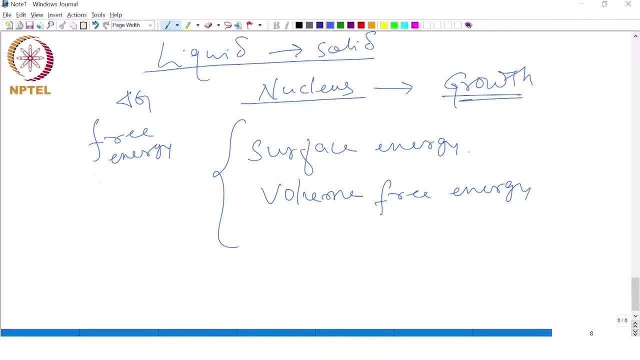 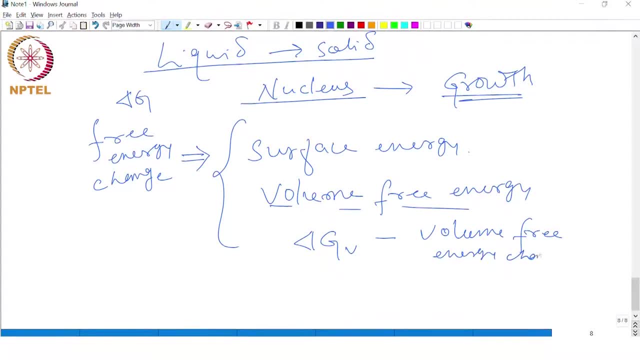 And gamma be the surface energy per unit area, then, considering this nucleus as a spherical particle, we can write this delta G in terms of delta G, v and the gamma. So, if you consider the 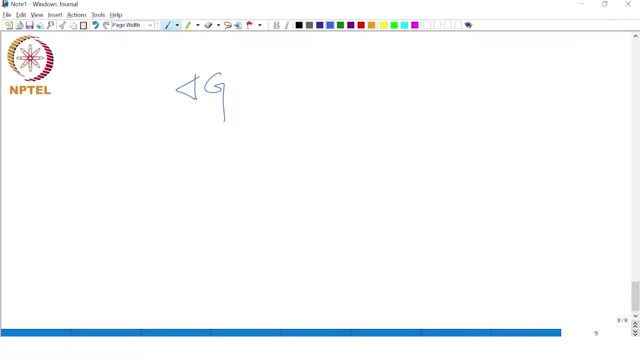 nucleus to be spherical. the volume will be this if you take the radius as r. So therefore this will be the total volume, free energy change and the surface energy would be this: Where 4 pi r square is the surface area right and these two components of delta G. that means 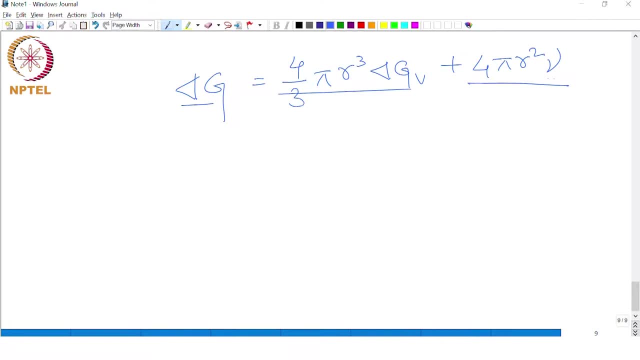 this one, and this can also berepresented graphically where you plot it in terms of the surface area. You can also smaller the size or the radius. this is delta G positive and this is negative. So you will get the particle size or the radius of delta G right. So, in particular, 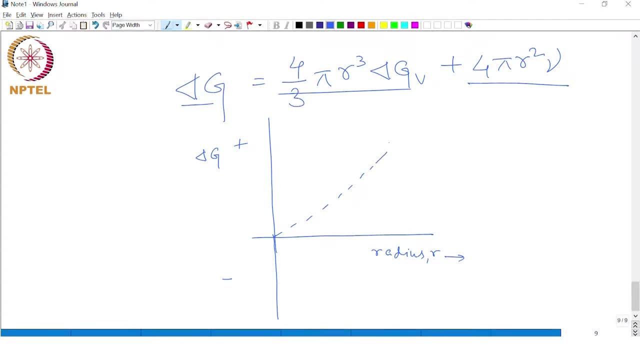 this is the radius. here we can give it as delta G and this is the radius. So if delta This is the surface area contribution and this is the volume free energy contribution, which is negative, And the summation of these two is delta, delta. 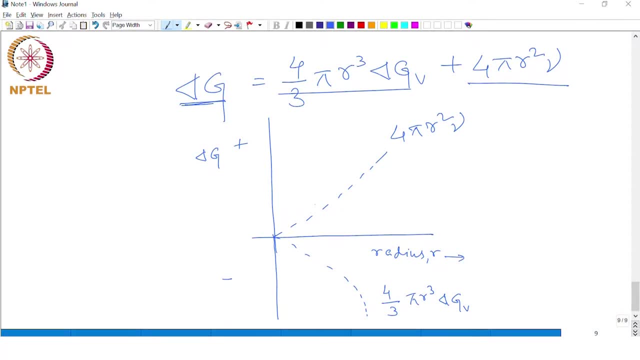 g, which can be shown here as the sum of these two, Is like this: ok, So if you take this maxima here, the maximum, this is the critical size of the nucleus. ok, So if the size of the nucleus does not attain this size, it will. 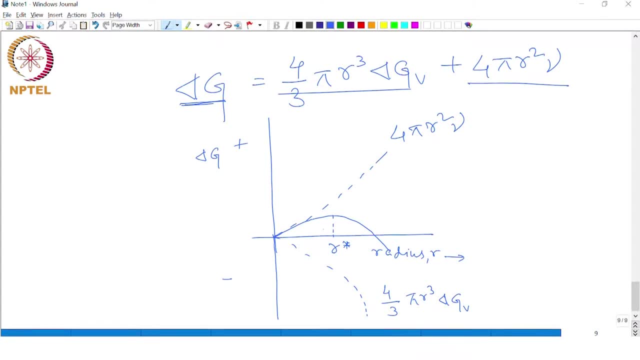 dissolve back into the liquid and will not grow as a solid right. So the nucleus has to attain this critical radius. Then only it is going to grow right. So since it happens at the maximum, this d delta g dR is 0, bank. 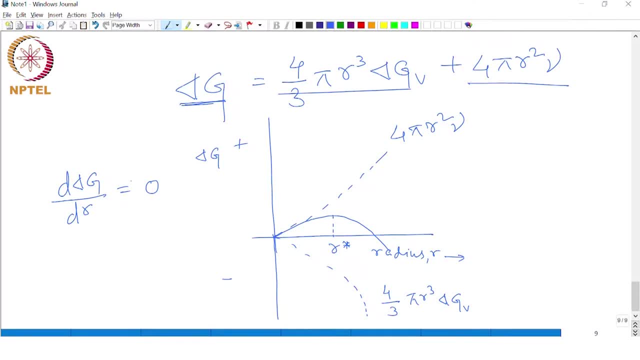 3,ол and 0.. 0, 0, zero, d, d, d, 0. So if you differentiate this you get it. So this is equal to 0 and from here you can derive the critical size of the nucleus. 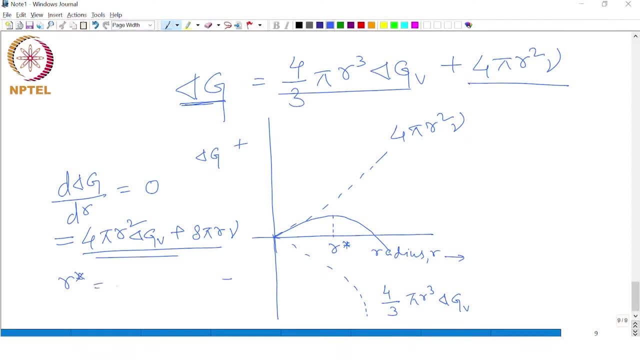 which will come out as minus 2 gamma by delta g v. ok, So the The negative sign here indicates that this delta g v is negative. That means the free energy, the volume free energy, will reduce once it attends this critical size, right? So 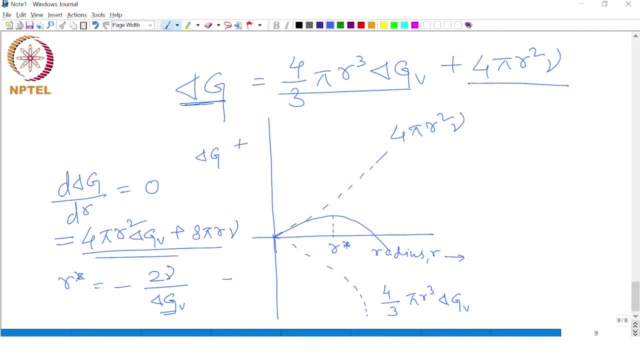 that is what the negative sign indicates, And similarly the corresponding delta g value will be given as: